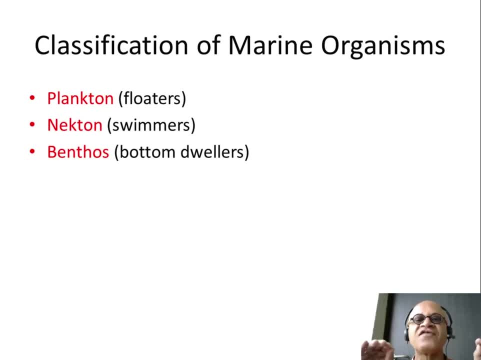 because many of the planktors have some kind of, say, appendage or buoyancy chamber that allows them to go up and down or move, change directions. okay, but mostly they are floaters. they move with the currents, okay. 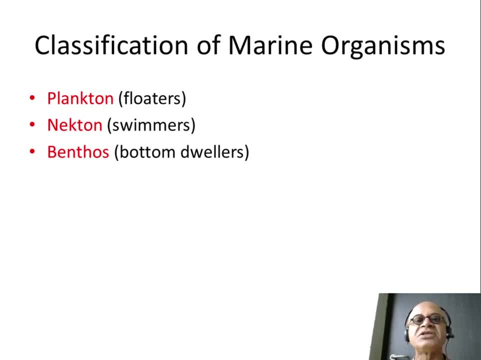 Nekton are swimmers. they have explicit appendages that allow them to change direction, move forward and dive and so on and so forth. so we'll see that most of the fish will belong in this category. and benthos is the bottom dwellers. they are on the bottom of the ocean, so in the coastal ocean the bottom is very close to the surface. 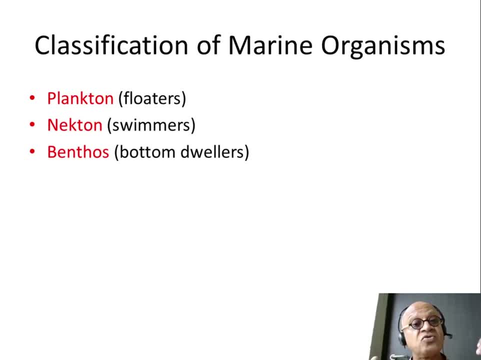 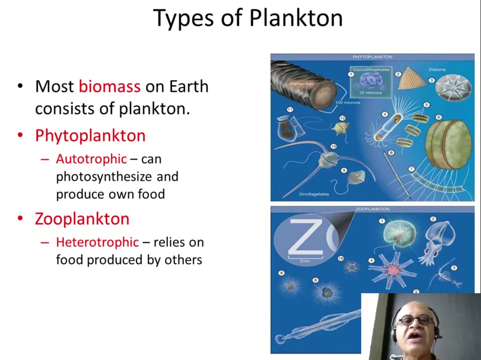 and the deep ocean is several kilometers deep right. so we have seen oxygen profiles, light. we will see again light. it's very dark, very high pressure, very cold water and yet there is a lot of life at the bottom of the ocean. and we'll also see how biodiversity or the number of species changes in the open ocean versus the coastal ocean versus the bottom of the ocean, and so on. okay, so types of plankton here we have. most of the biomass on earth consists of plankton. why? because actually primary production in the ocean. 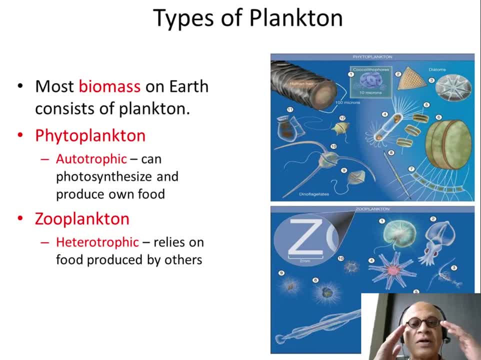 serves as the base of the food chain for most of life on earth, even though we don't all directly eat fish. in many ways, plankton serve as the base of the food chain, and ocean covers 75% of the earth's surface and there is a lot of space for phytoplankton, for example, to grow and zooplankton to grow to eat them. right, so already used phytoplankton. phyto is light. 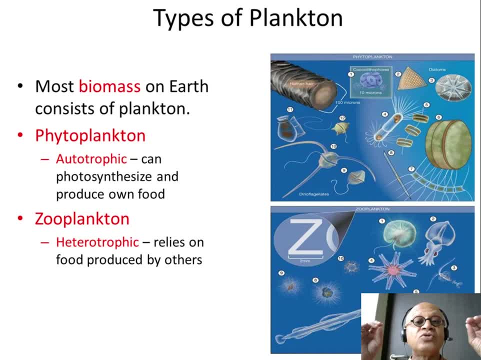 basically a drifter that has ability to use light, to photosynthesize, is called phytoplankton. it's an autotroph, it can produce its own food and zooplankton, or zooplankton is a heterotrophic, relies on food produced by others. so there is a size reference given here of 100 micrometers, 10 to the minus 6 meters. 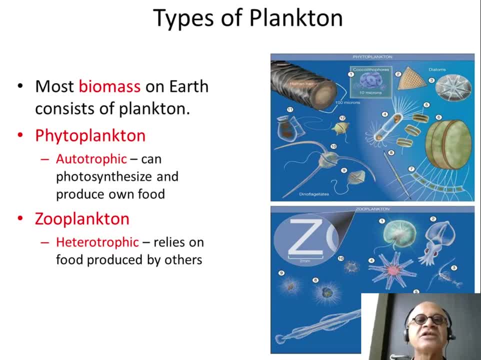 9.146 meters. examples of phytoplankton, things that use light to photosynthesize include things like coccolithophores, which are merged into a cluster here. there are multiple coccolithophores in this. these are kinds of diatoms, all these. these are kind of dinoflagellates. okay, just terminology. you don't have to remember all of them. 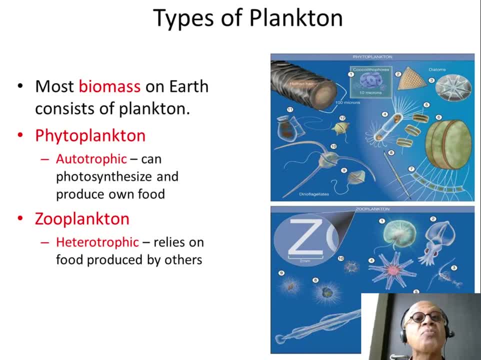 all these. these are kind of dinoflagelltes. okay, just terminology, you don't have to remember all of them. Coccylexophores form calcium carbonate shells and diatoms typically form silica shells and dinoflagellates have soft material. 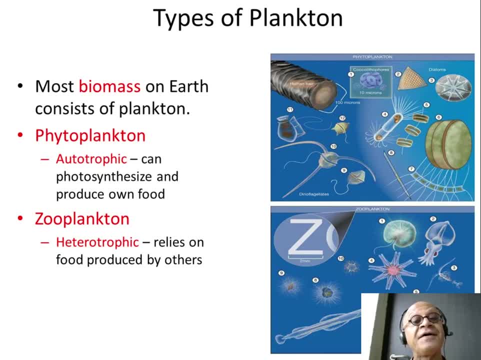 It turns out that when we talked about paleoclimate and determining past climates, the shells that are either calcium carbonate or silica can go drop to the bottom when the phytoplankton dies or being eaten and spit out, And they store the information about the climate because when they are formed at the surface, the temperature and so on. 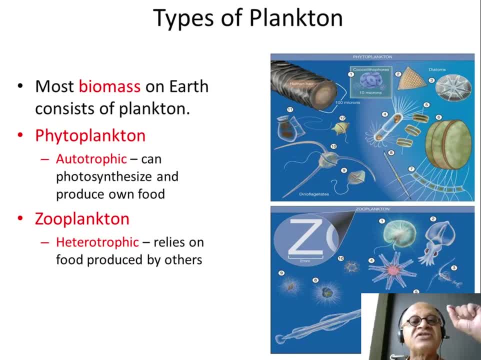 That's right. Salinity et cetera can affect the crystal structure of the calcium carbonate or the silica, and the abundance of these phytoplankton shells also can say something about the circulation. Okay, So these are called paleoproxies or proxy thermometers and so on. 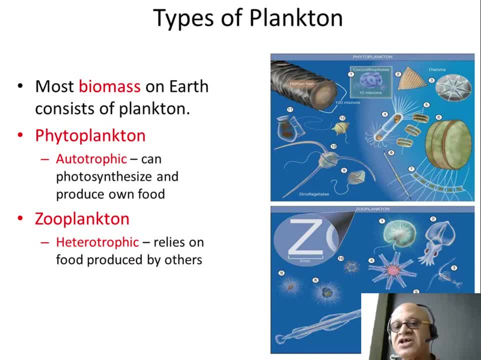 Okay, Very cute, right. So these are the zooplankton examples. These are kind of various things: Larvae of the jellyfish. This is the larvae of something else. This is like a copepod. This is a larvae of a fish. 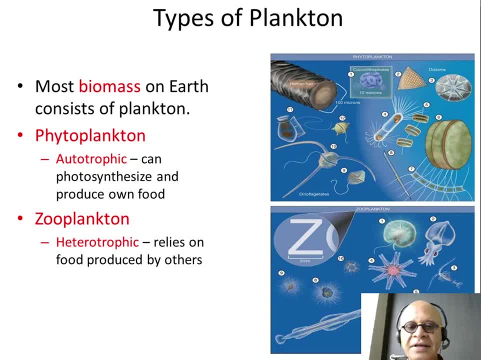 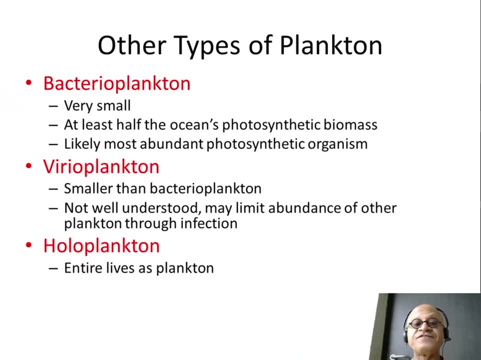 This is an arrow worm. I think this is the. I don't know, You don't need to remember all the names, But these are the zooplankton. They are heterotrophs. Okay, Other types of plankton. 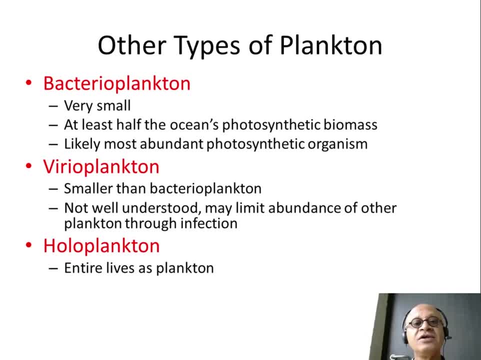 There are bacterioplankton, which are very small. These are at least half of the oceanic, The ocean's photosynthetic biomass- and there are virioplankton. Yes, there are many, many, many trillions of viruses in the ocean. 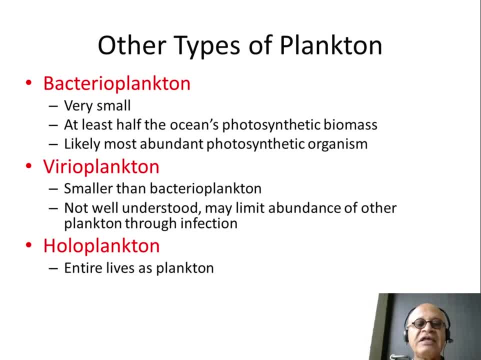 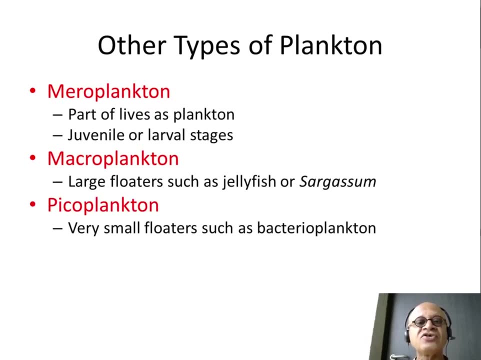 And what are called holoplankton, which live their entire life as plankton, which means they always remain in the water column. They never use the bottom or any kind of surface. Why do we say that? Because there are others which are miroplankton. 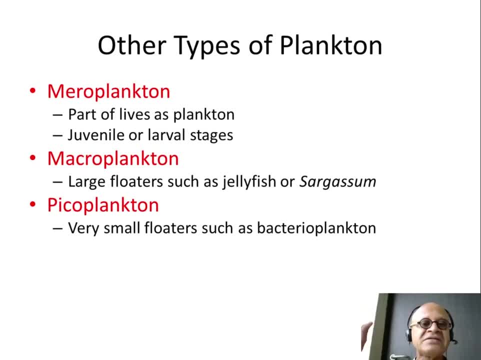 So they are. Part of their life is spent as plankton in juvenile or larval stages, But they are attached to something at some stage in their life. Macroplankton are large floaters like jellyfish or sargassum, which is found in the Atlantic Ocean. 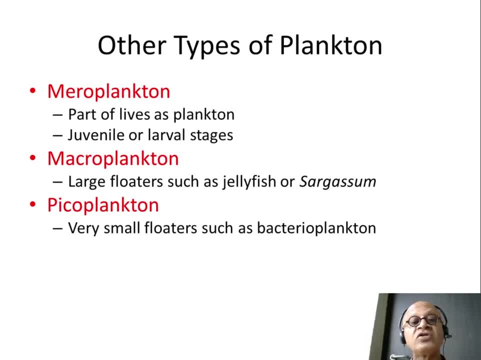 It's a kind of a weed seaweed, And also size can be used. It's microplankton, picoplankton, nanoplankton and so on. So you have holoplankton, miroplankton and macroplankton, picoplankton and so on. 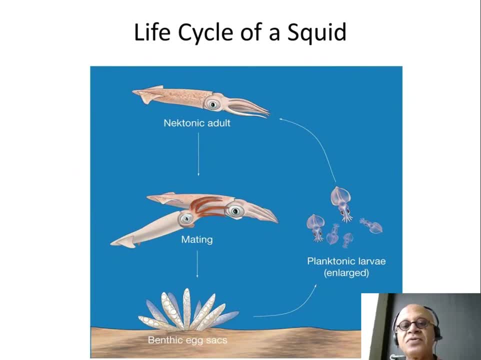 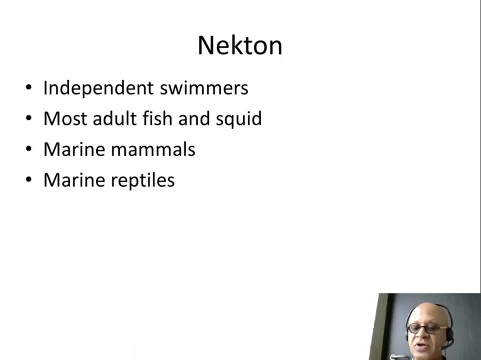 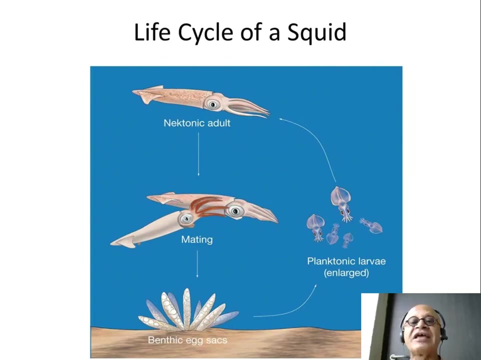 So here is an example. The adult squid starts as a benthic organism when it's in its egg form as an egg sac. Once it hatches it becomes a planktonic larvae. There is the mating to produce the egg sac which is attached to the bottom. 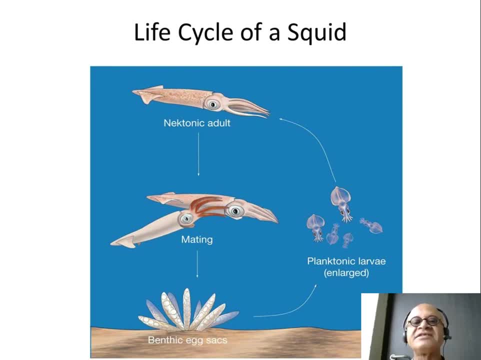 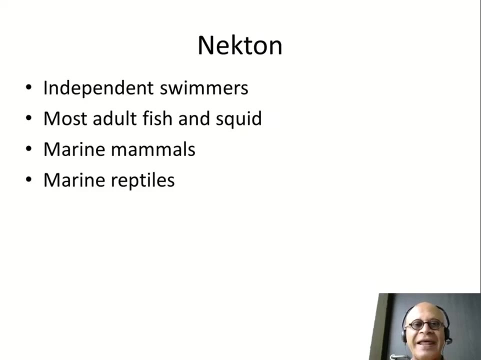 And then it becomes a nektonic adult, which means as an adult it can manipulate its movements using its tentacles and the gill structure in the back. So it is a species that is not plankton all its life It's a miroplankton. 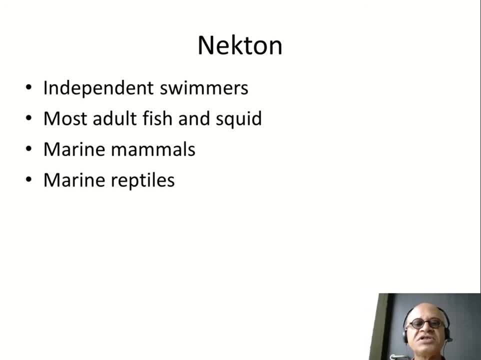 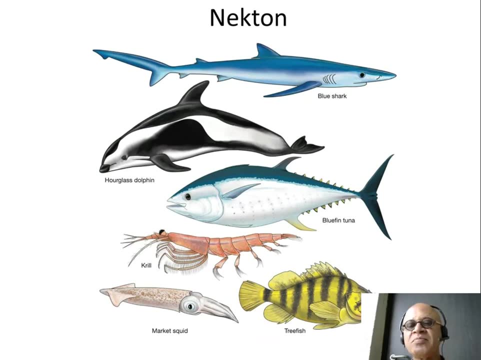 Nektons, independent swimmers, most adult fish and squids, marine mammals, marine reptiles and so on. So here is it. Examples: blue shark, hourglass dolphin, bluefin tuna, krill, market squid and tree fish. 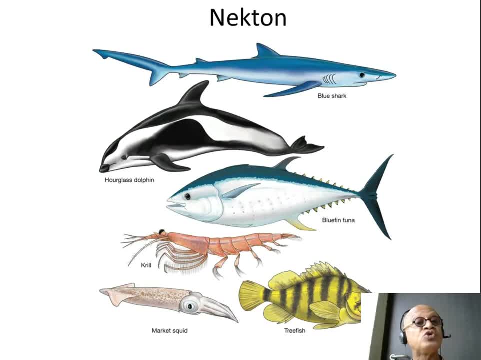 There are many interesting stories for, let's say, bluefin tuna, for example. It's one of the most efficient and fast swimmers. It never sleeps To create oxygen. it has to constantly keep moving to ingest new water to get more oxygen.